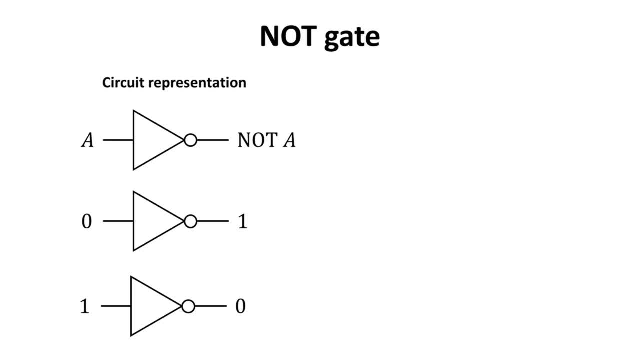 of the NOT gate, also known as the inverter, which implements logical negation. In other words, this gate transforms a 0 into a 1 and vice versa. The logical relationship between the input and output of a gate can be summarized in: 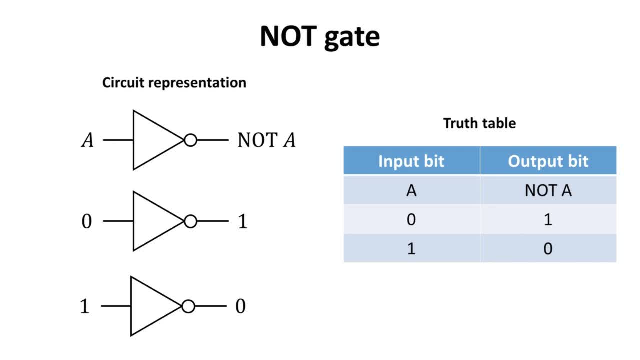 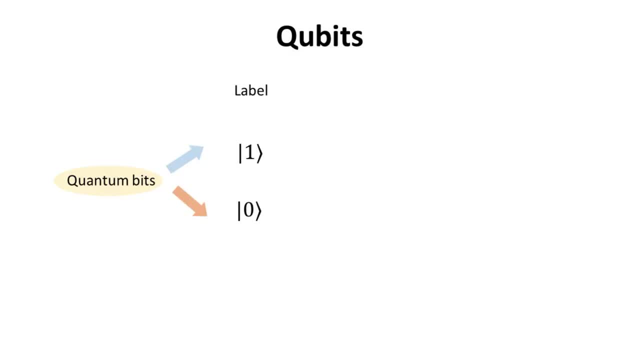 the form of a truth table, as shown, which identifies all possible input combinations and the output for each Quantum. bits or qubit, on the other hand, are labeled as ket 0 and ket 1.. The brackets enclosing the 0 and 1 are called kets, which 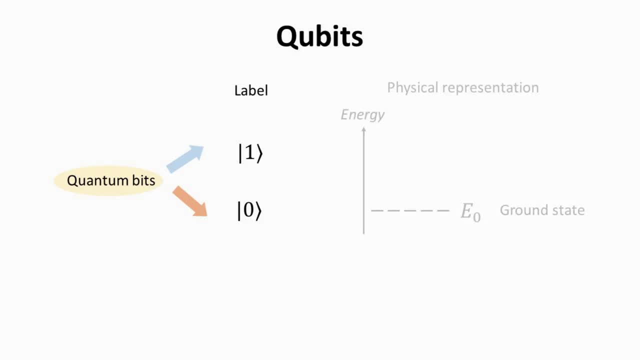 is a notation to represent the number of the input and output of the gate. The bracket, on the other hand, is a notation to represent quantum mechanical states. The ket 0 state corresponds physically to the lowest energy state of a two-level system. 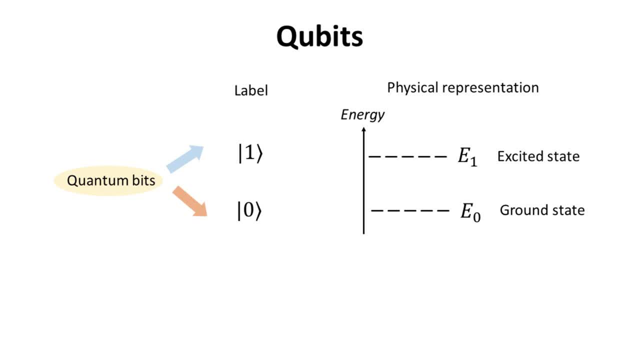 also known as the ground state. On the other hand, the ket 1 state corresponds to the excited state. The energy difference between these states, delta E, needs to be gained or lost in this exact discrete amount in order to change the state from one to the other. 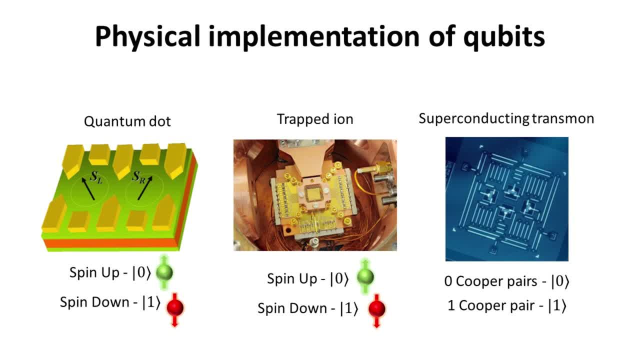 Physically, the two-level quantum system can be the spin of electrons confined in quantum dots, or that of trapped ions, as shown, or it could also be the presence and absence of cooper pairs in superconducting systems, among many other types of qubit platform. 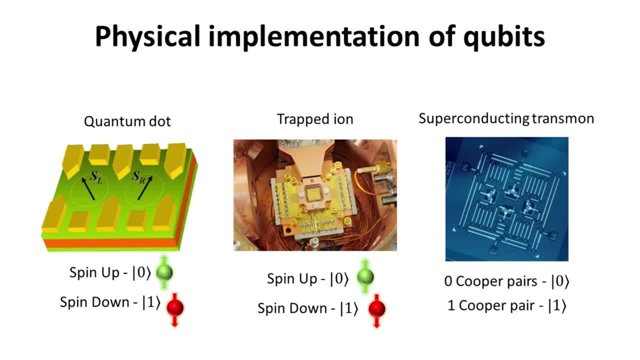 We shall defer to future videos the discussion of these various physical implementation of quantum computing. Just like its classical analog, qubit can be made to be a quantum system. but it can also be a quantum system. In other words, qubit can be made to be a. 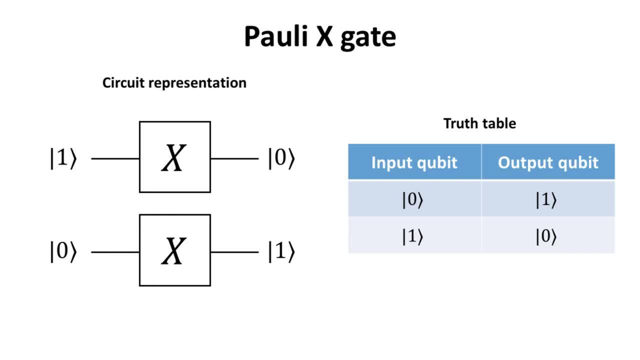 quantum system, Just like its classical analog qubit can be made to be a quantum system. Just like its classical analog qubit can be made to be a quantum system. Just like its classical analog qubit can be made to be a quantum system. 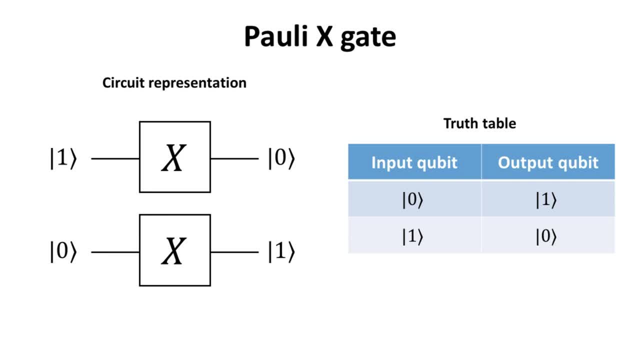 The quantum counterpart of the classical NOT gate is the Pauli X gate, which turns the ket 0 into the ket 1 and vice versa. In what follows we shall introduce the different types of single qubit gates, their mathematical representation and its operation on the qubit. 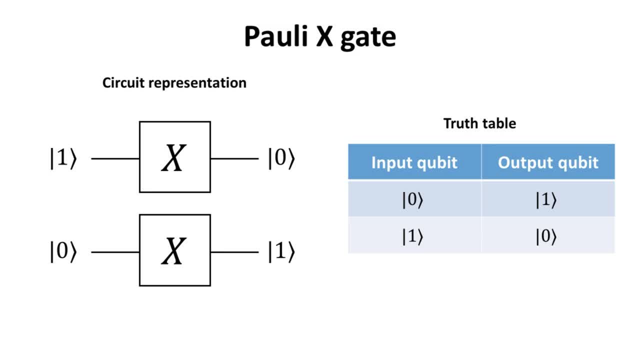 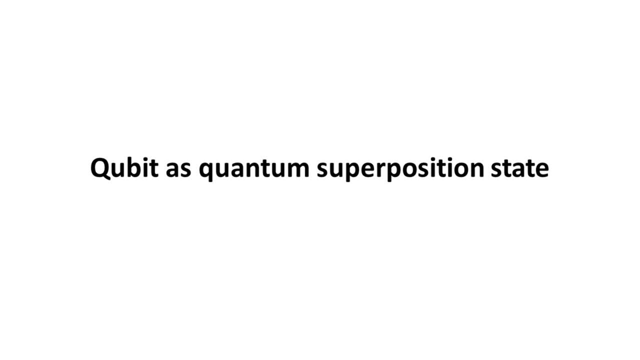 We shall defer the discussion of their physical implementation to future videos. Part 2. Qubit as Quantum Superposition. Part 2. Qubit as Quantum Superposition state. Qubit are fundamentally different from the classical bit. One of the property that sets qubit apart from a classical bit is its ability to be. 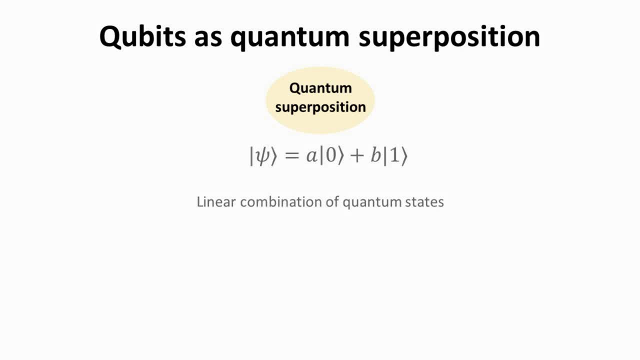 in a superposition of ket 0 and 1.. A general qubit state is represented by the ket psi as follows: where psi is a linear combination of ket 0 and ket 1.. The numbers a and b are complex-valued. 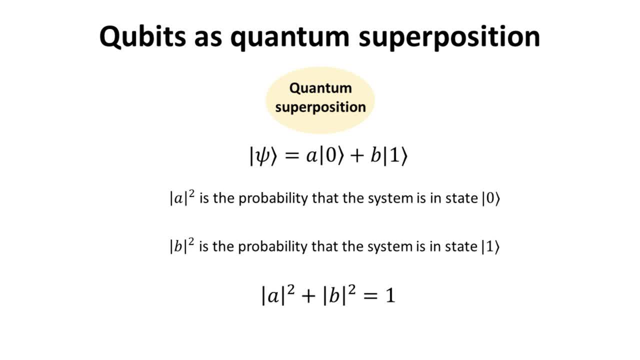 The square of the modulus of a and b yields us the probabilities that the system will be in the state ket 0 or ket 1 respectively. Since they are probabilities, they have to add up to 1, which is also known as the normalization. 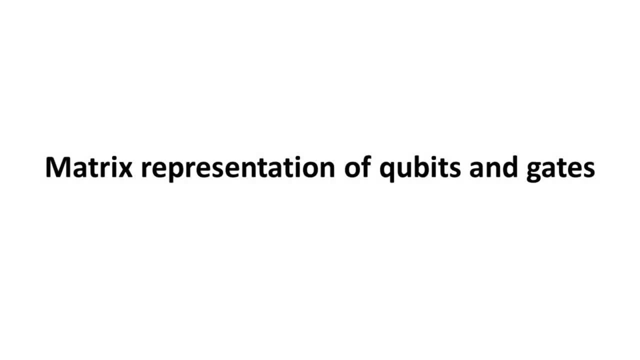 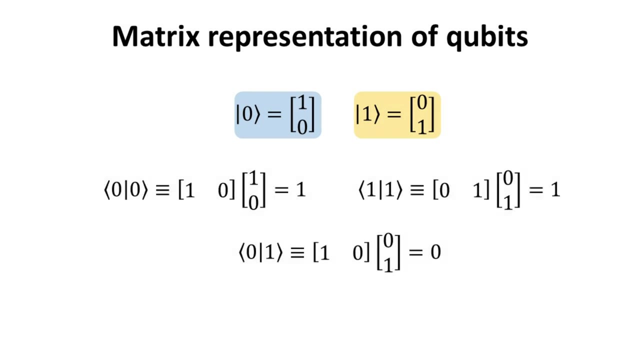 condition Part 3. Matrix Representation of Qubit and Gates. Mathematically, the 0 and 1 kets can be represented as 2-dimensional column vectors as shown. It is straightforward to see that they form an orthonormal basis set which any state vector. 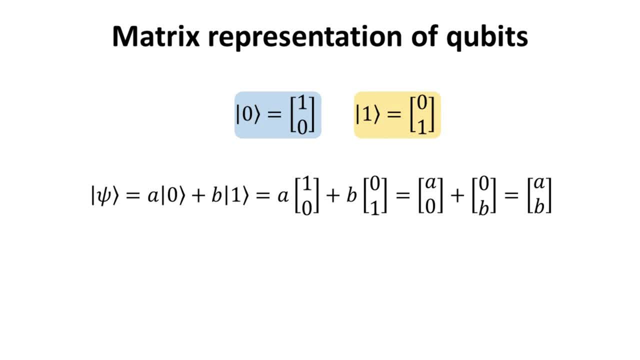 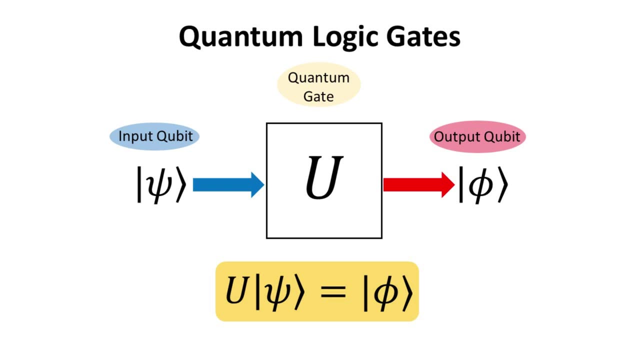 psi in can be represented as a linear combination of these basis states. We say that 0 and 1 kets span the 2d Hilbert space, which is the vector space of 2-dimensional complex-valued vectors where the qubit live. 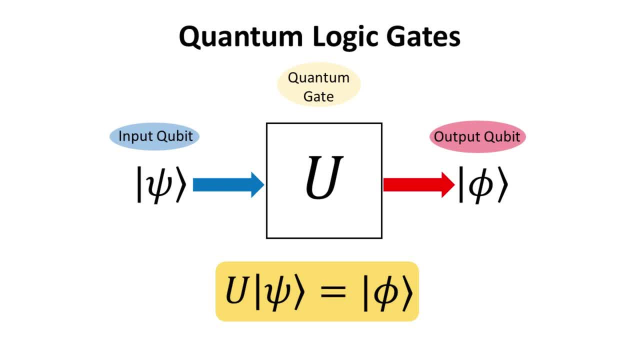 The quantum logic gates which operates on the qubit are represented by 2x2 matrices, herein denoted by U. They are also known as operators in quantum mechanics. Mathematically, the action of the quantum gate on the qubit, psi, is given by U times the 2x1 ket vector. 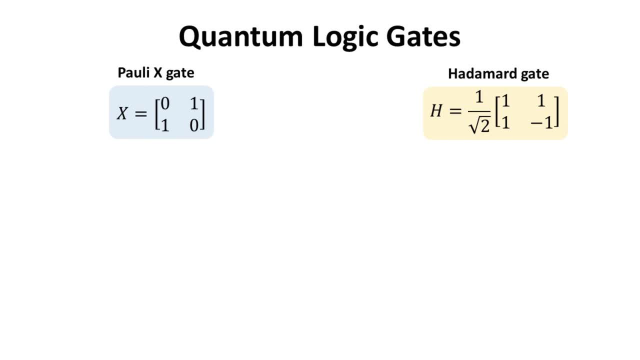 Let's consider two of the most common quantum logic gates: the Pauli x gate and the Audemars H gate. Their matrix representation are as shown. We see that the action of the x gate on the 0 ket turns it into 1 ket. 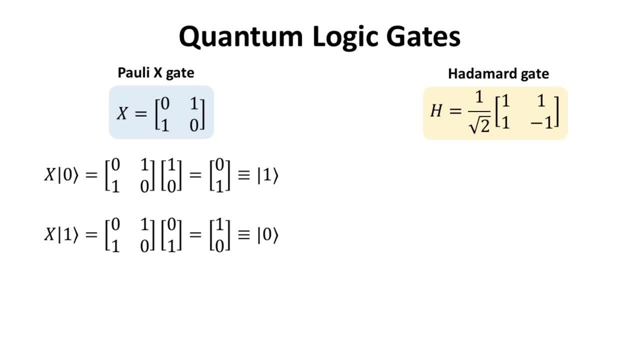 Thus the Pauli gate is analogous to the inverter For a general qubit psi. the x gate exchanges the complex coefficients A and B, The Audemars gate H. on the other hand, when applied to the 0 ket. 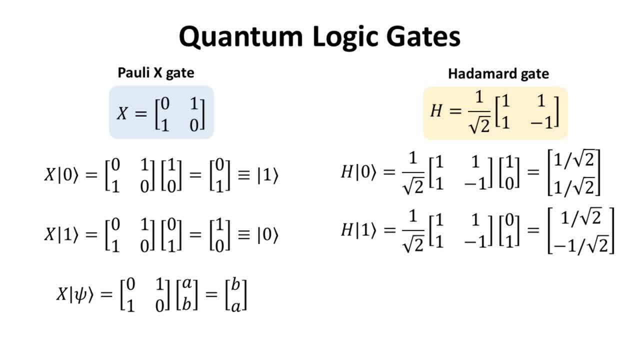 creates a superposition state with equal amplitudes for 0 and 1 kets. The same happens when the H gate is applied to the basis state 1, except now with a relative minus sign in one of the amplitudes When the H gate acts on a general qubit, psi. 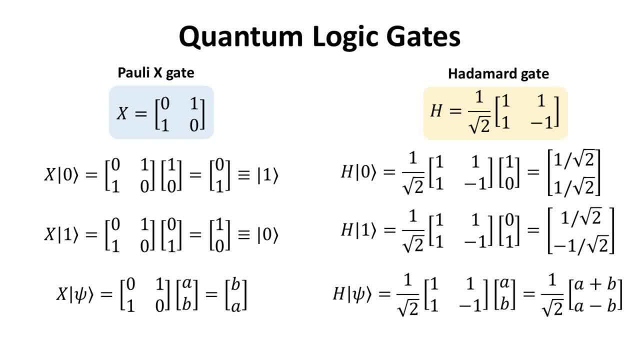 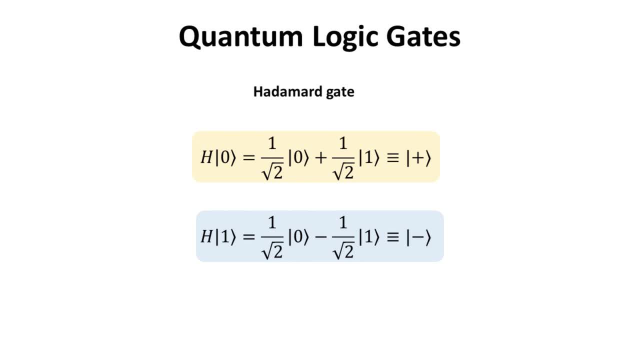 it mixes the components to be an equal weighted sum or difference of the two. as shown, The two resulting qubits bits from the H gate application are also known as the plus and minus kets, which are equal weight superposition of the two basis states. 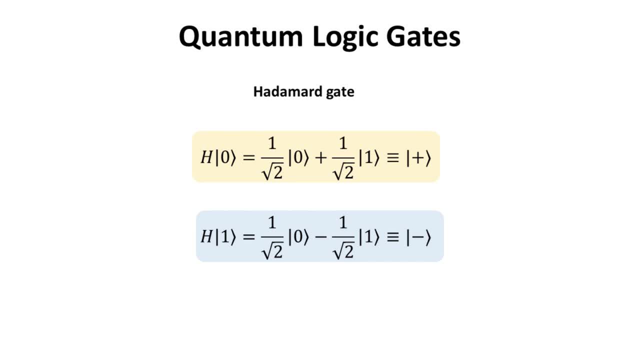 Thus we see that the H gate brings the qubit into a superposition of the two basis states. Quantum logic gates cannot be any 2x2 matrix. They must have two important properties. First, they have to be Hermitian matrices. 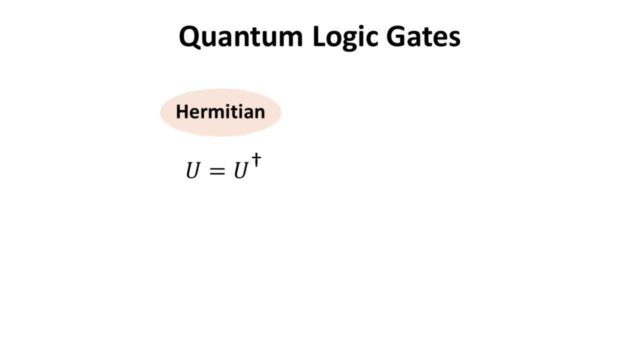 where the matrix is equal to its own adjoint. The adjoint of a matrix is its transposed complex conjugate. They also have to be unitary, which means the matrix multiplication of the operator with its own adjoint is equal to the identity matrix. 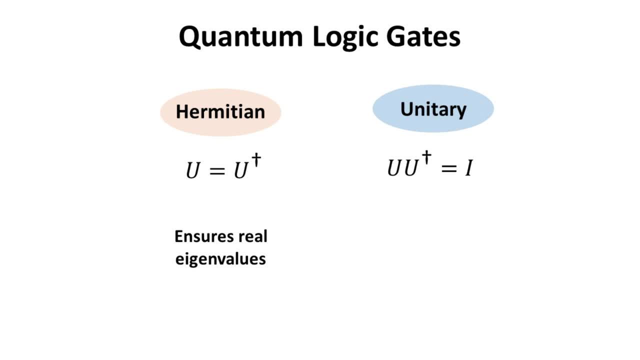 The first requirement ensures that the eigenvalues, also known as the observables, are real valued. The observables are measurable quantities, so they must be real in order to have any physical meaning. On the other hand, the second requirement ensures the complex conjugate. 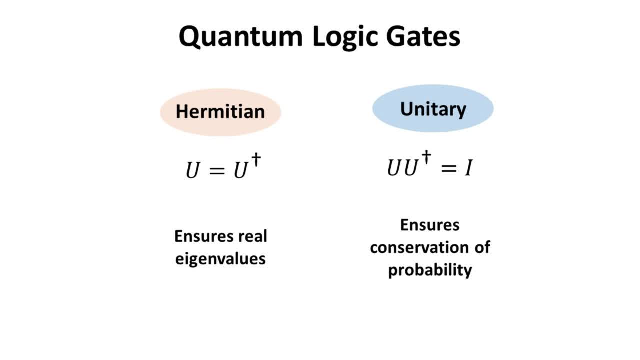 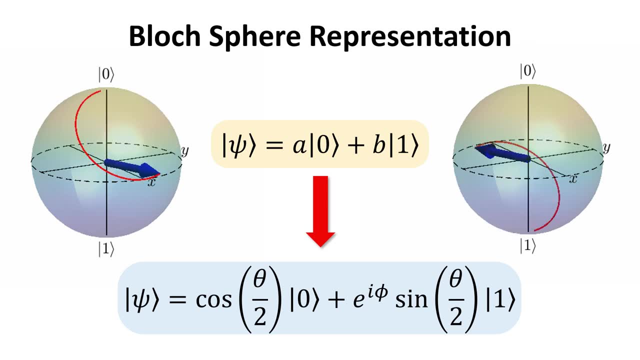 which is the conservation of probability. In other words, no qubits are leaking into or out of the systems. Before we proceed, we would like to add another utility to our toolbox. It turns out that one can faithfully map the qubit state onto a geometrical block-sphere representation. 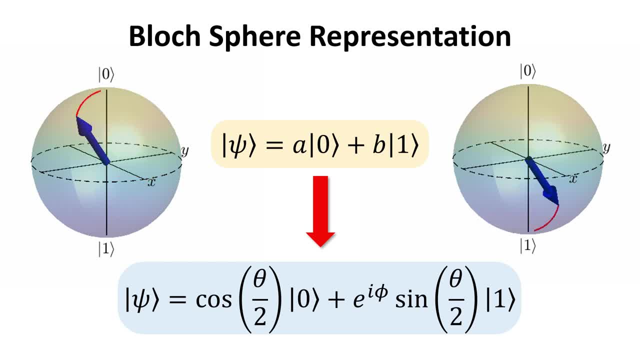 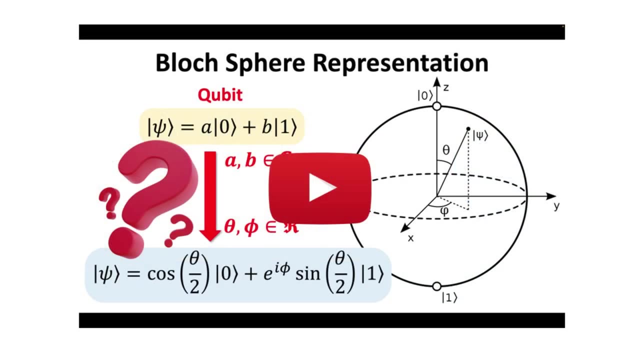 In other words, the two complex amplitudes A and B can be mapped onto the geometrical variable theta and phi, where theta and phi are the usual polar and azimuthal angles in spherical representation. The block-sphere provides a powerful visualization of the state of a qubit. 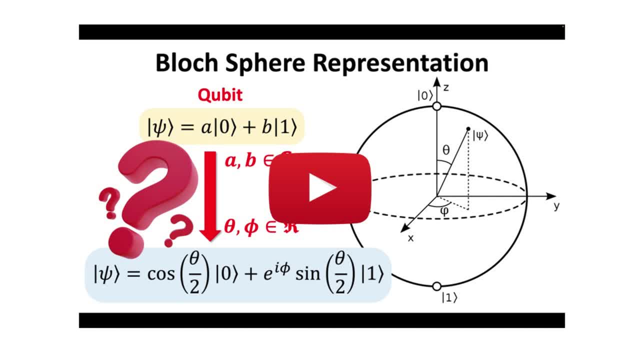 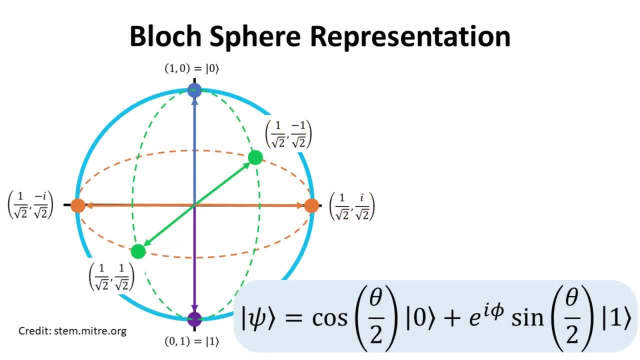 and is a powerful tool for understanding quantum mechanics and quantum computing. You can refer to this video in the same playlist. for its derivation In the block-sphere representation, the zero ket will be located at the north pole, while the one ket at the south pole. 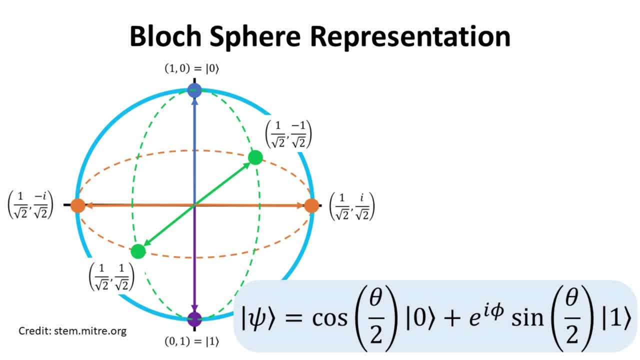 All states with equal weight superposition of the zero and one kets are located along the equator as shown. The operation of any single qubit gates can then be represented as mapping from one point on the block-sphere to another, as we shall demonstrate in what follows. 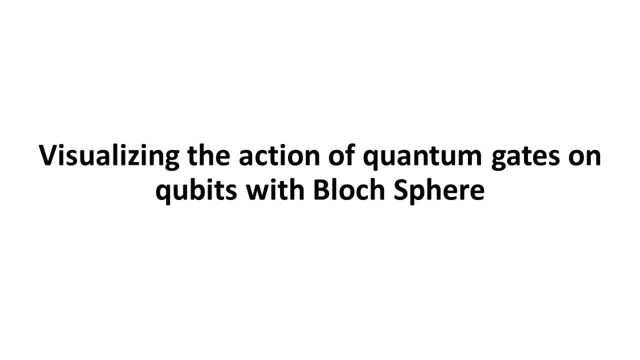 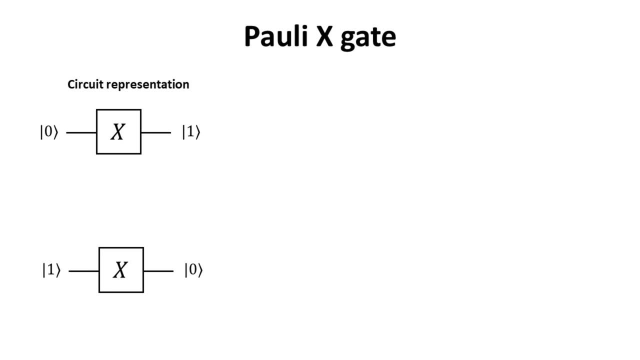 Part 4: Visualizing the action of quantum gates on qubits with block-sphere. Armed with the block-sphere representation, let's explore the Pauli x-gate operation on a qubit. We recall the matrix representation of the x-gate and its operation on zero and one kets. 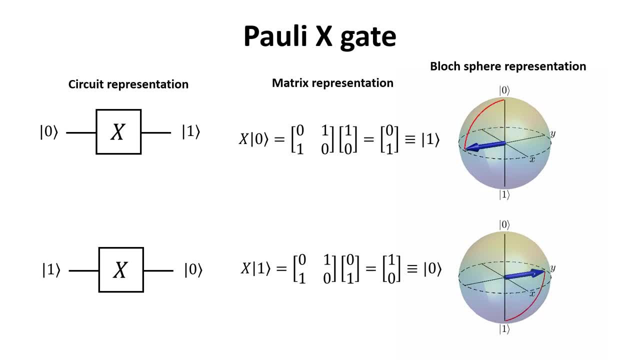 In the block-sphere representation we see that the x-gate simply maps the initial qubit state onto the opposite pole, say from zero ket to one ket and vice versa. In the block-sphere illustration we see that the action of the x-gate is represented by a rotation of pi with respect to the x-axis. 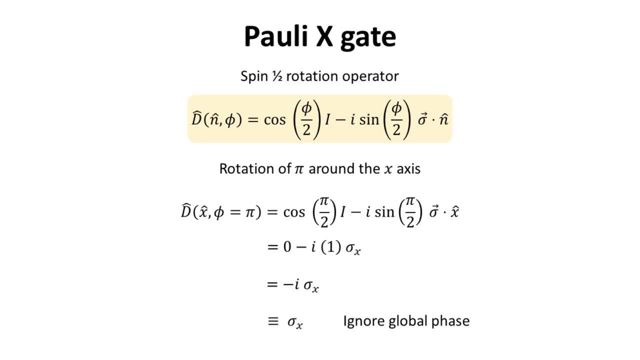 This is not an arbitrary choice. Using the definition of the rotation operator for spin one-half systems, we can show that the x-gate is exactly the same as the rotation of pi with respect to the x-axis. In the last step we have removed the minus i factor because it is just a global phase. 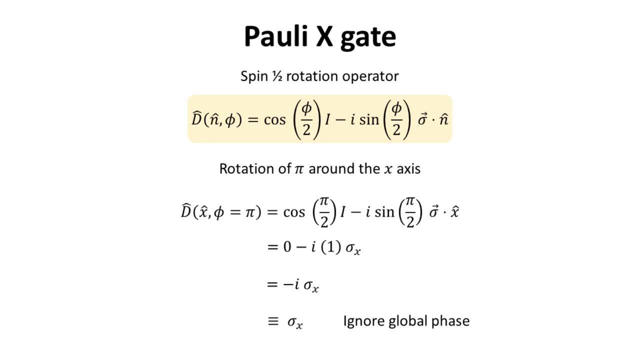 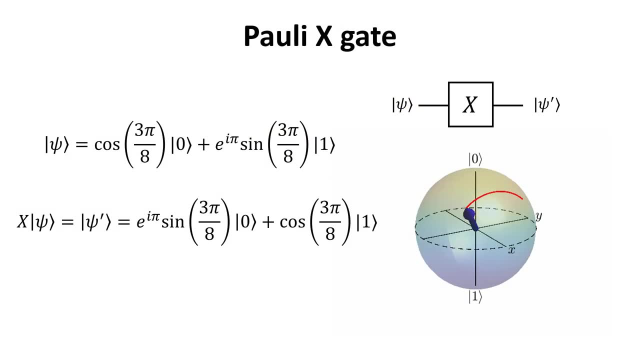 Recall that in the block-sphere representation all qubit that differs by a global phase lies at the same point on the surface of the block-sphere. Here's another example of the x-gate operating on a more general qubit, psi. Note that the trajectory traces out a half circle. 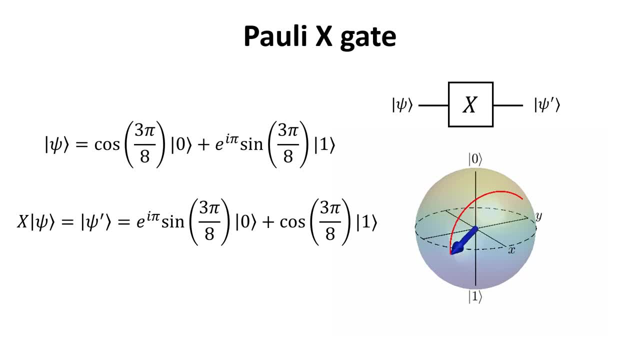 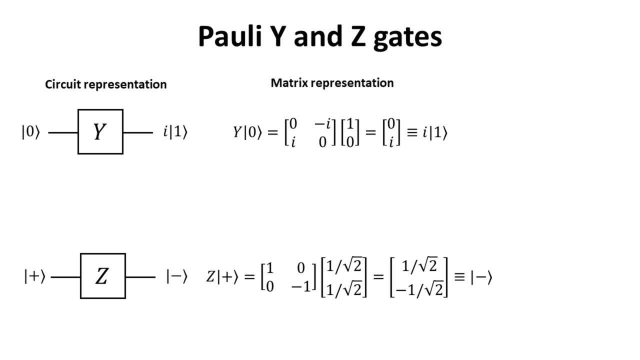 in accordance with the pi rotation with respect to the x-axis. In similar fashion, one can also define the y and z Pauli gates as rotation of pi with respect to the y and z-axis respectively, Per the general definition of the spin one-half rotation matrices. 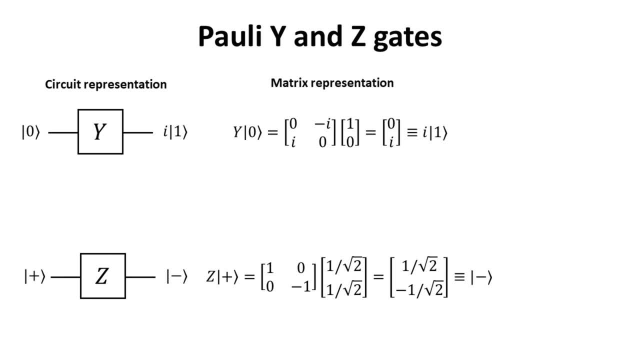 one can also check that these rotations correspond to the Pauli matrices, sigma y and z. Their operations are illustrated on the block-sphere. The y-gate rotates the zero ket by pi with respect to the y-axis, ending up as the one ket. 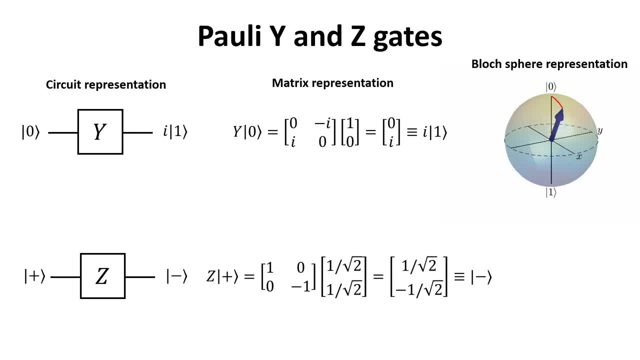 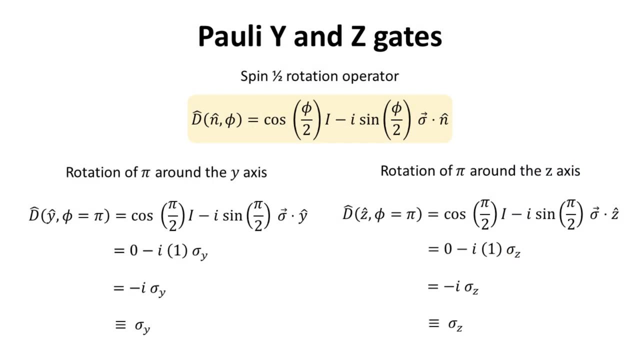 Note that a global phase is incurred during the operation, which can be dropped. The z-gate rotates the plus ket by pi with respect to the z-axis, ending up as the minus ket, Using the general definition of the spin one-half rotation matrices. 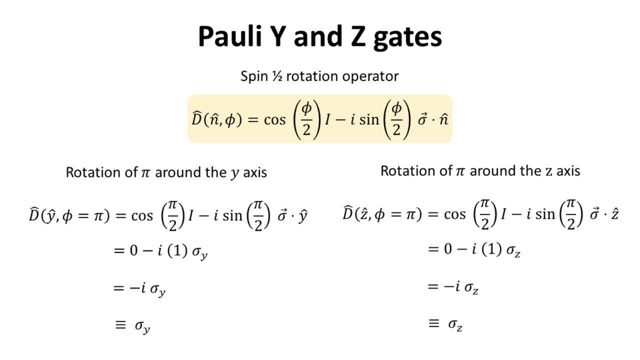 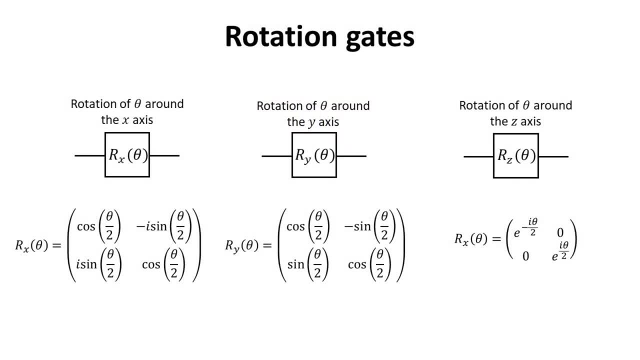 one can also check that these rotations indeed correspond to the Pauli matrices sigma y and z. Feel free to pause if you would like to inspect the math. Thus, by extension, the Pauli x, y and z gates can be generalized to rotation gates. 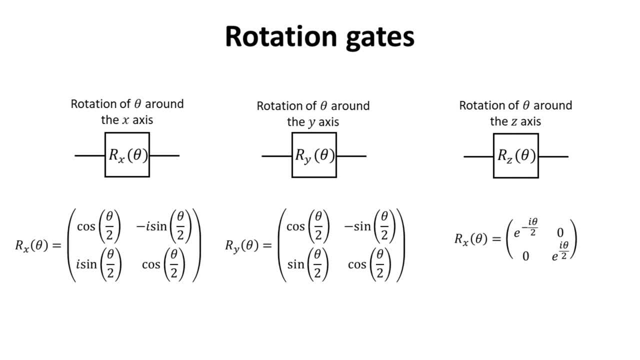 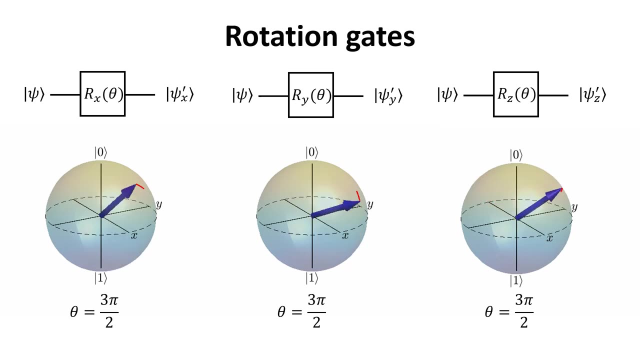 which performs rotation at arbitrary angle theta. instead, Their respective matrix representations can be obtained from the general spin one-half rotation matrix. We illustrate here the respective rotation gates operation on the block-sphere with the angle theta equals to 3 pi over 2.. 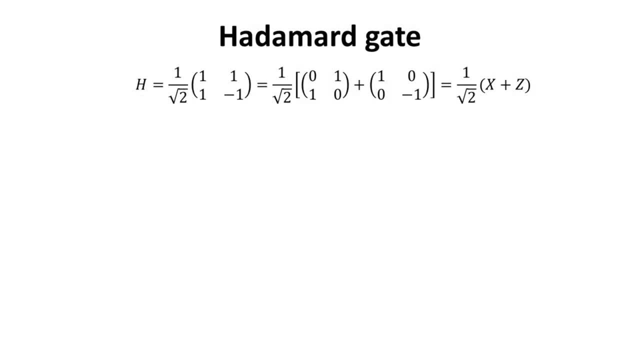 By now. we hope that we impress upon you that the single-qubit gate operations are just rotations on the surface of the block-sphere. We shall end with a last example, the Audemars H-gate, From the matrix form of the H-gate. 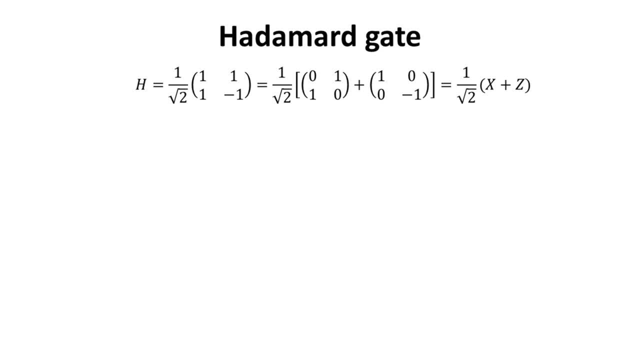 it is easy to see that the H-gate is a linear combination of the x and z gates. We seek to find the rotation angle phi and axis n in the spin one-half rotation matrix that yields the H-gate Expanding out the dot product. 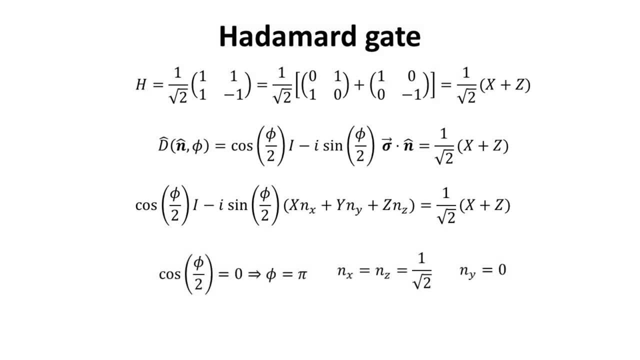 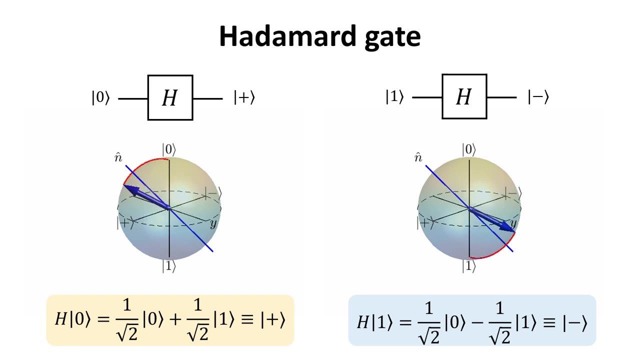 and comparing both sides of the equation, we can deduce that the angle phi is equal to pi and the axis is lying diagonal on the x-z plane, as expected by the form of the H-matrix. With this we can illustrate the H-gate operation on the block-sphere. 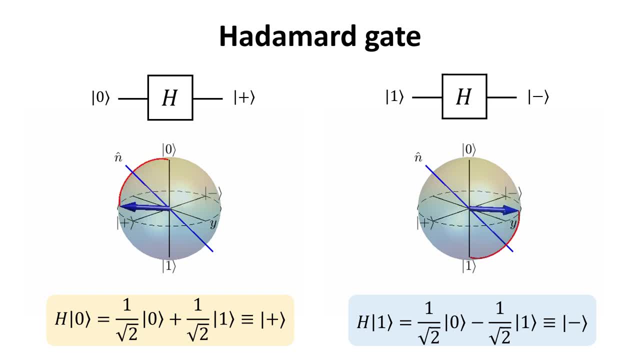 It is a rotation by pi around the blue axis n which is pointing diagonal in the x-z plane. The H-gate, acting on the zero ket, brings it to the plus ket, while its action on the one ket brings it to the minus ket. 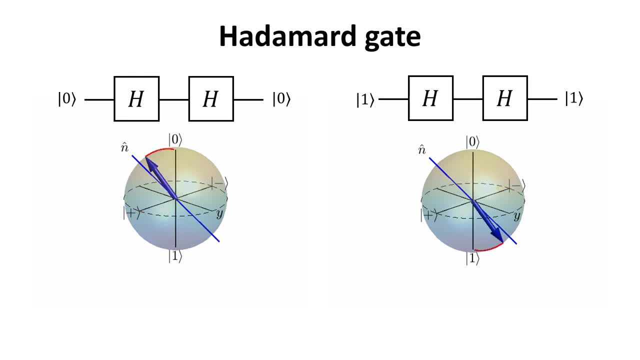 Two successive applications of the H-gate would therefore take the initial zero or one basis state back to its original state, as it would give a rotation of 2 pi around the same axis. We can also verify this through its matrix representation. Recall that the H-gate is Hermitian and Unitary. 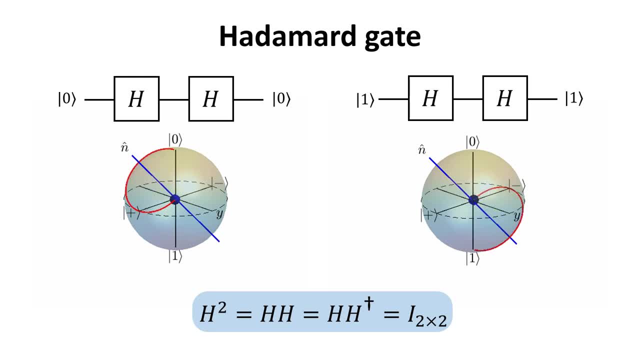 Since it is Hermitian, it is equal to its own transpose conjugate. Since it is also Unitary, the product of itself, with its transpose conjugate, is equal to the identity matrix. Therefore, the application of two successful H-gates leaves the initial qubit unchanged.